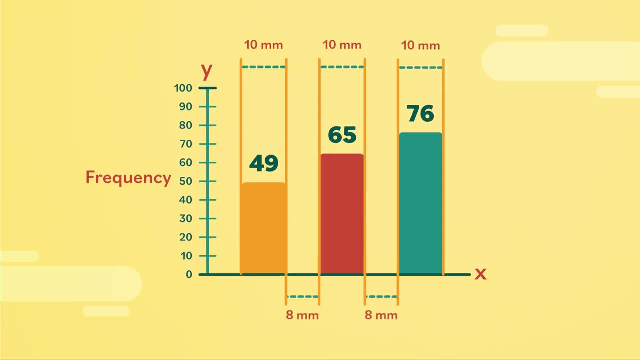 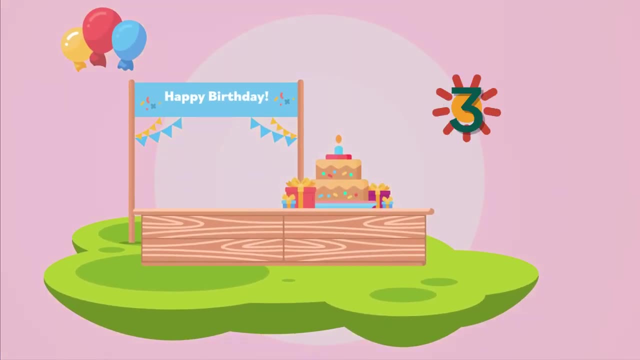 it's important that the width of the bars is the same, as well as the space between each one. For example, Daniel's having a birthday party and his mom wants to offer three different flavors of ice cream. She can't decide which flavors to buy. 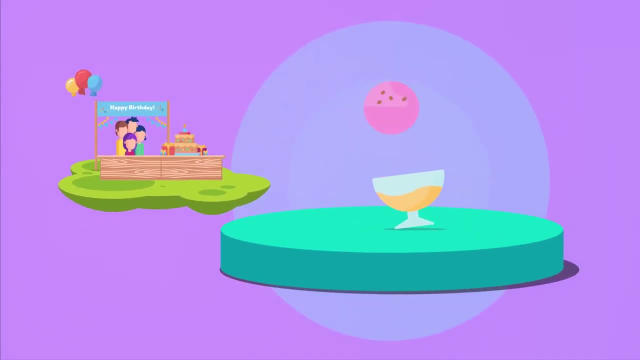 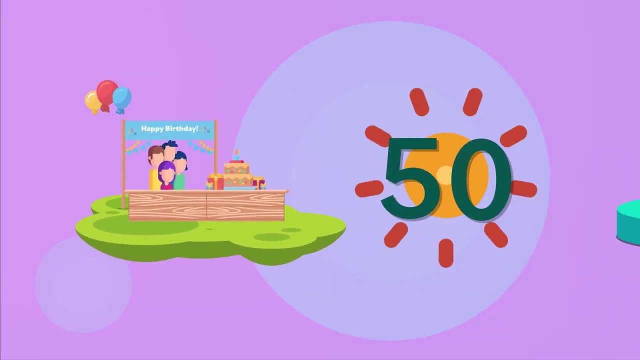 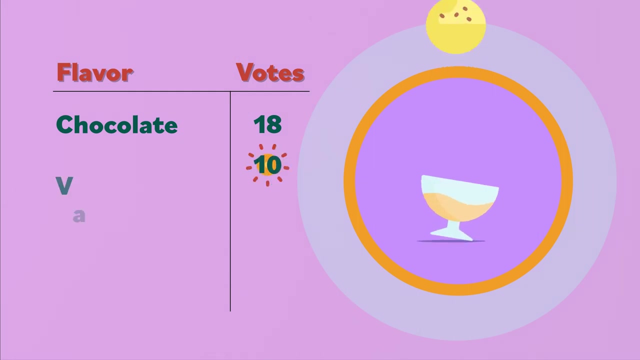 so she asks the guests what they prefer: Strawberry, cotton candy, vanilla, mint or chocolate. After getting responses from 50 people, she organizes the data into a table. 18 people voted for chocolate, 10 for vanilla, 8 for strawberry. 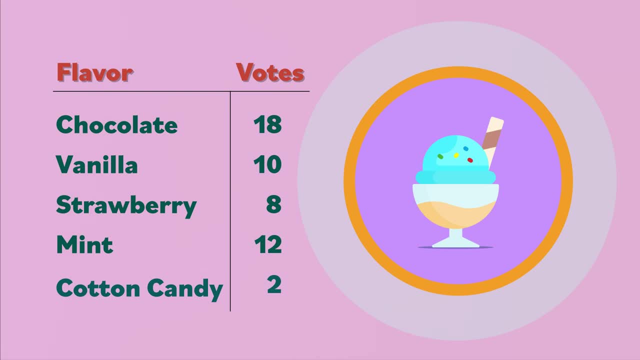 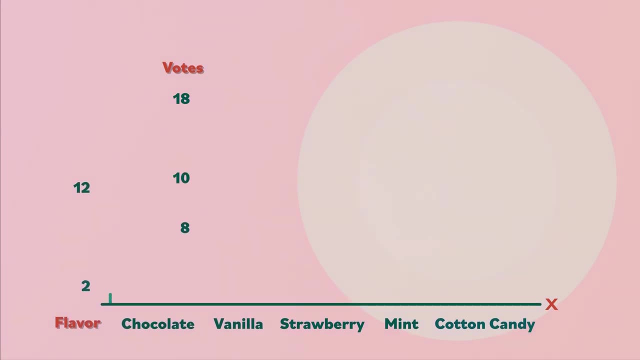 12 for mint and 2 for cotton candy. To make a bar graph, she lists each of the flavors on the x-axis and on the y-axis, the number of people who voted for each one, Since the largest number is 18,. 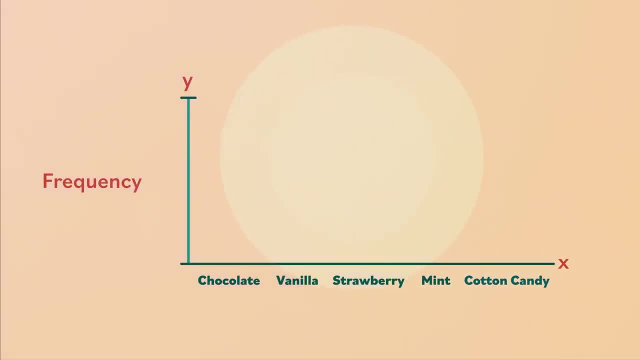 she uses increments of 2 on the y-axis, 2,, 4,, 6,, 8,, 10, until she reaches 20.. The key to choosing the increments on the y-axis is to consider the highest frequency. If you had 100 or 200 guests. 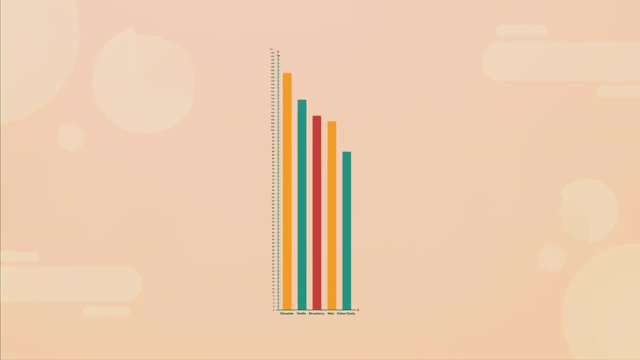 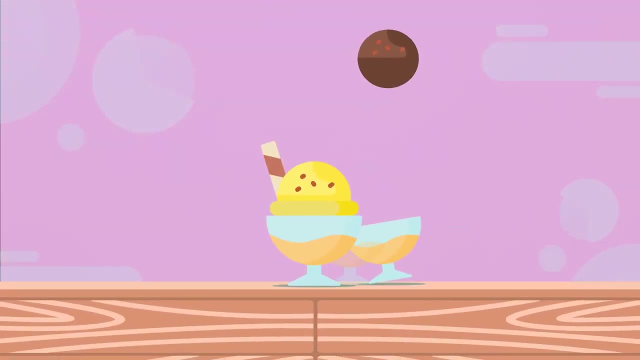 placing the numbers 2 by 2 would make the bar chart harder to read. With this chart, Daniel's mom can explain to her son that she'll be buying vanilla, chocolate and mint for the party, since these are the three flavors that are most popular. 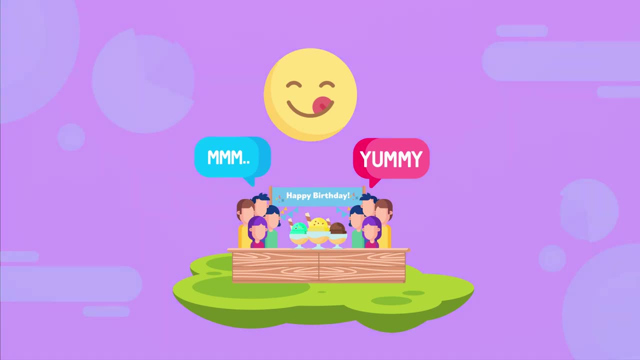 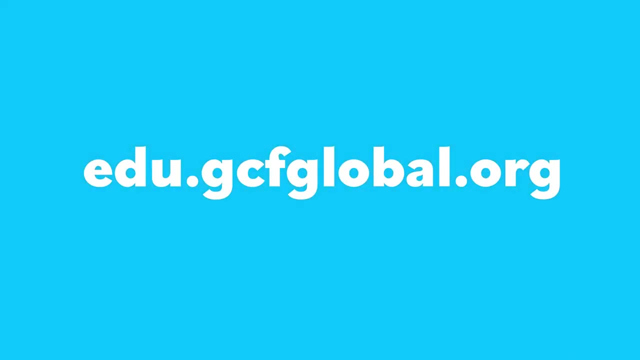 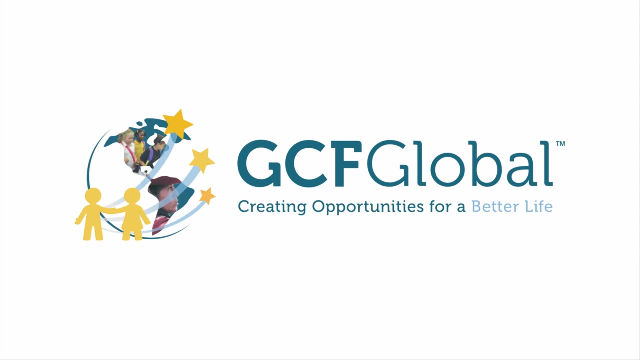 Feel free to check out our other videos about basic concepts and statistics or the full tutorial on our website at gcfglobalorg. GCF Global: Creating opportunities for a better life. 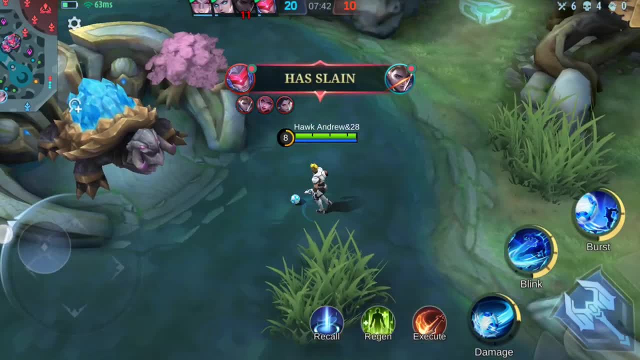 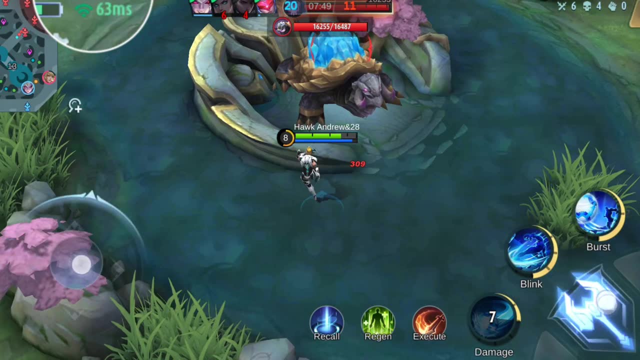 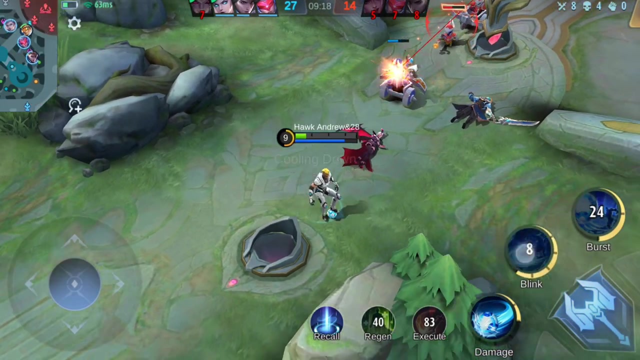 Is your mobile legends show you low and unstable ping while playing games. Recently, some mobile legends users have been complaining. unfortunately their internet is not stable. on their mobile legend, bang bang shows low ping and low ms while playing games. Now to solve your problem, watch this video to learn a quick way to solve internet not working.